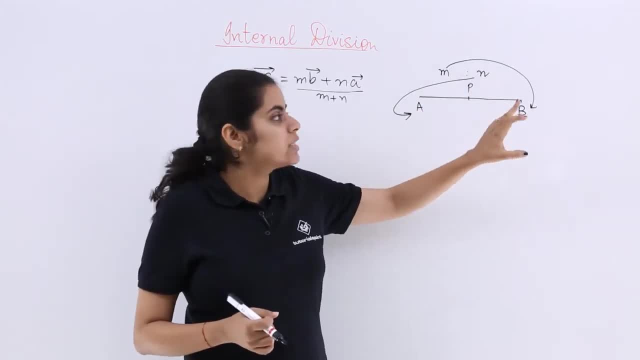 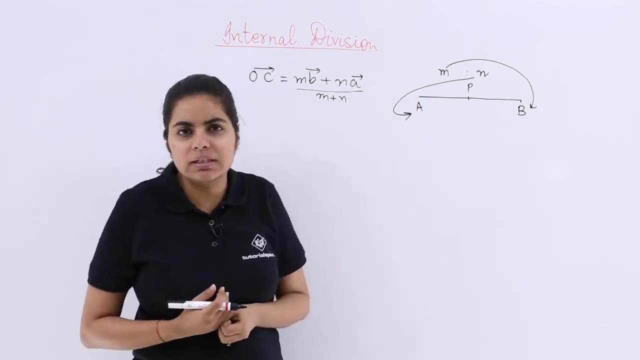 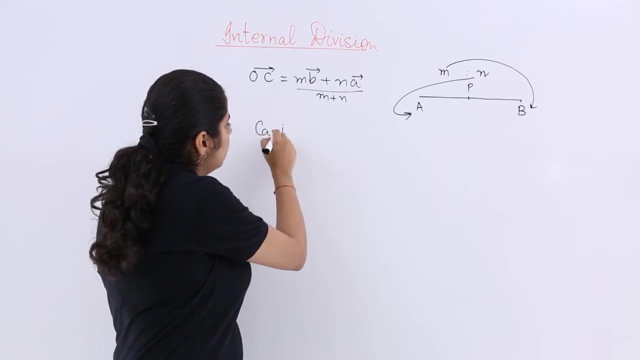 So what to do? You have to cross, multiply the ratios. I mean M with the farther one, N with the farther one, plus them in the denominator. Now certain cases are possible If I say that M and N, so I write case 1.. 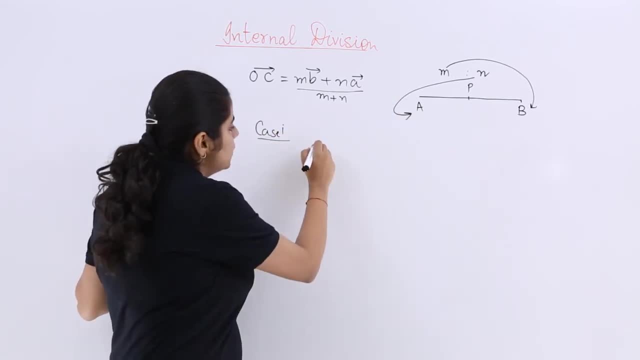 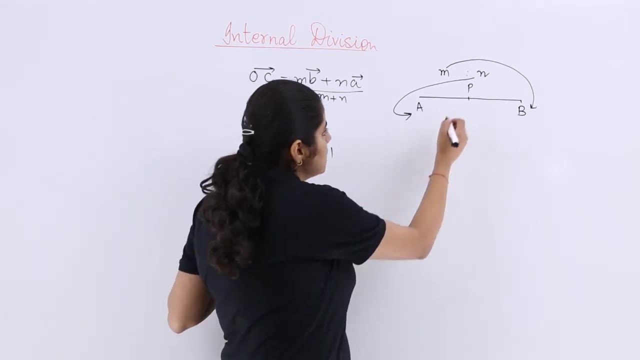 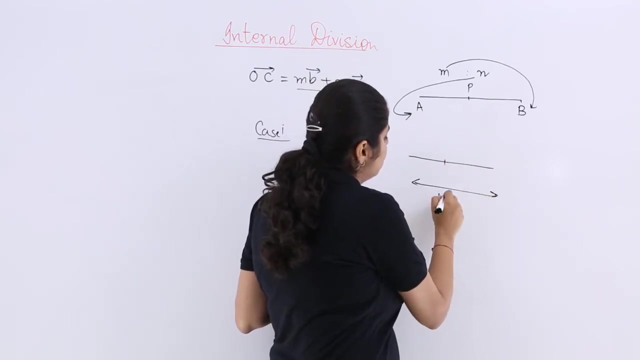 If I say M and N are 1 and 1.. So the ratio that has to be found out is 1 is to 1.. That means what That means. this P is exactly the midpoint, because if there is a line segment of 4 units and I say 1 is to 1 is the division. you know how to find out, Right. 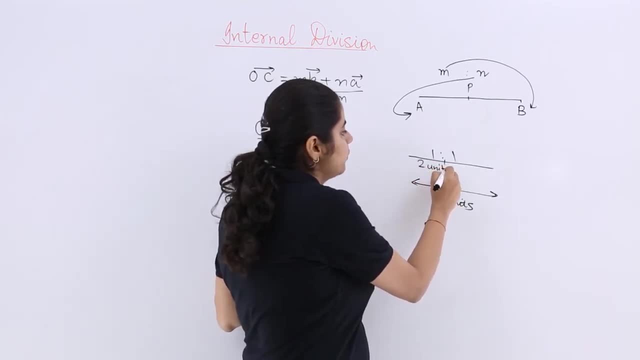 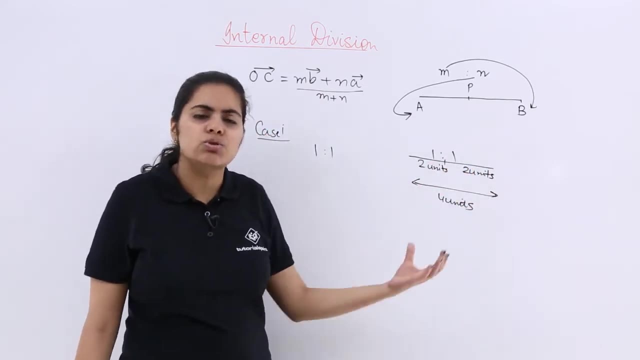 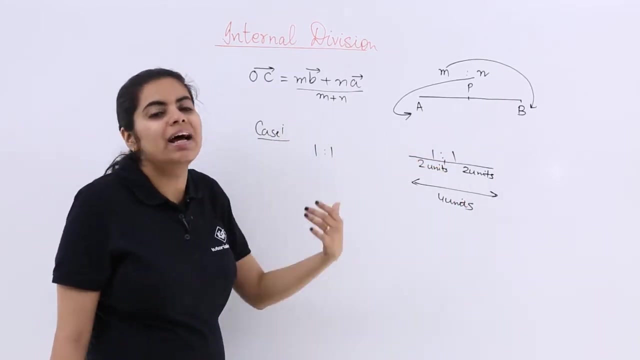 So that means this also should be 2 units and this also should be 2 units, Then only 1 is to 1 is possible and they add up to give 4.. So how to do that? Simply, in this particular formula you have to put value of M and N as 1 and 1 respectively. 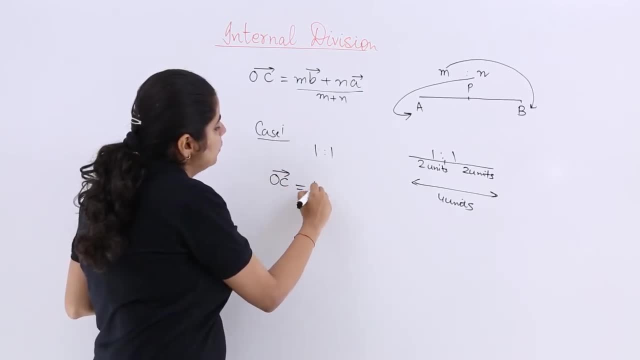 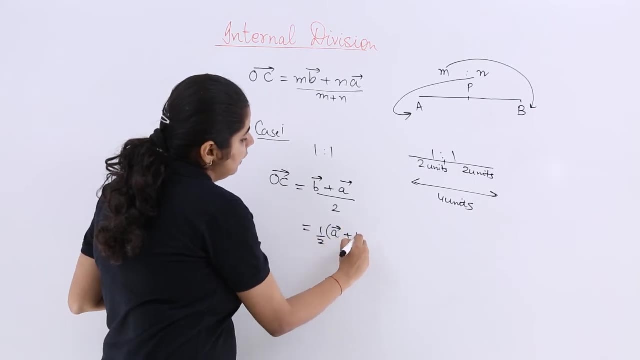 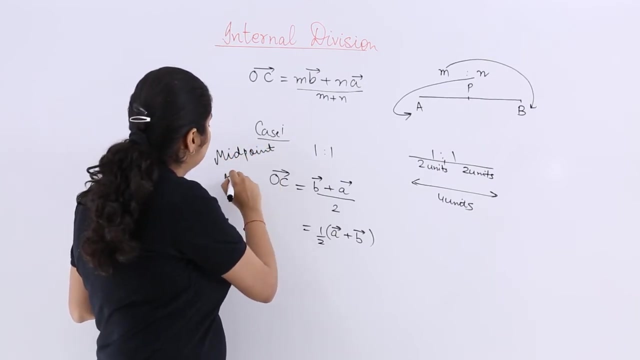 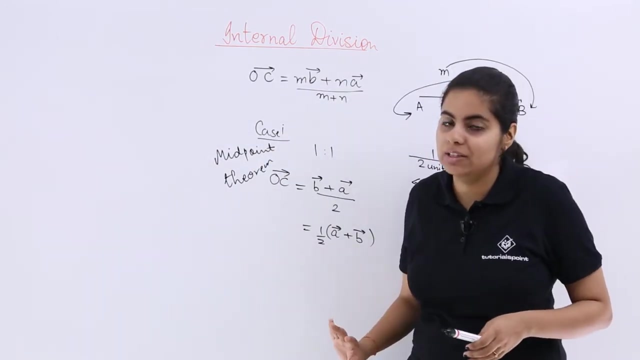 Then what should be the answer? Then OC vector is equal to B vector plus A vector upon 2 or half multiply by A vector plus B vector. So that is specifically called as the midpoint Theorem. Midpoint theorem you already studied earlier. Now we are studying in context through the vectors. 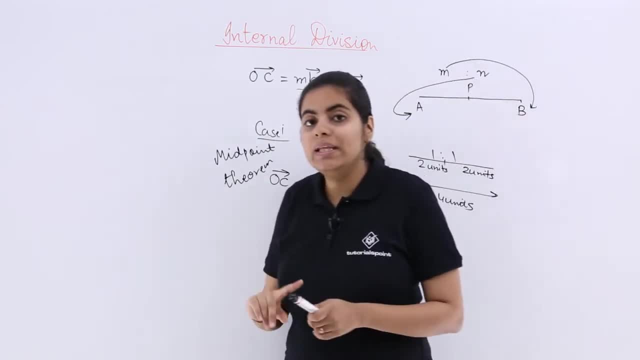 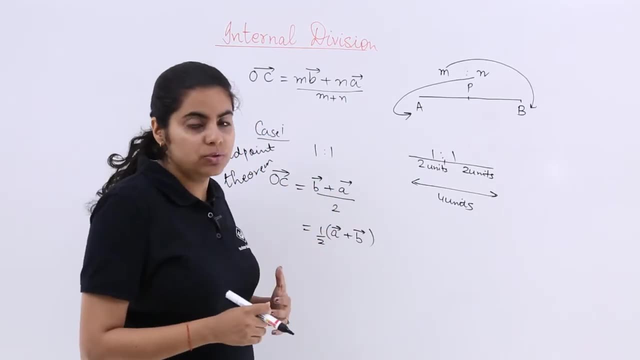 So that is how we study the midpoint theorem of vectors, with the help of the particular set formula that we have. The other thing which is very important is the second case that we talked about. The second case that we have to see is, you know, this is the particular formula. 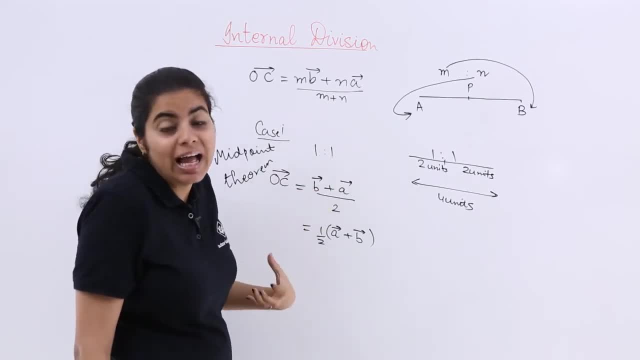 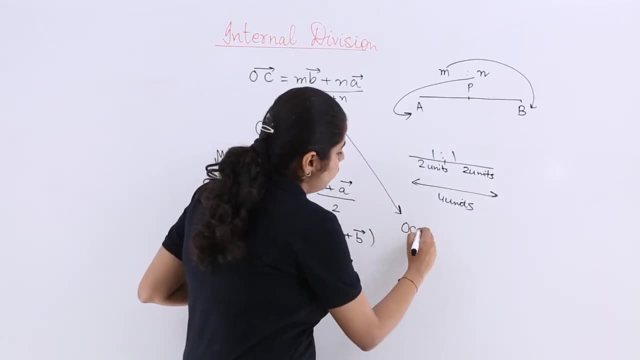 But what if I have to look to this formula with some other angle? That means, if I have to go into more, I have to go into more depth of this formula. So here I write the above step Now. OC vector is equal to MB vector upon M plus N. 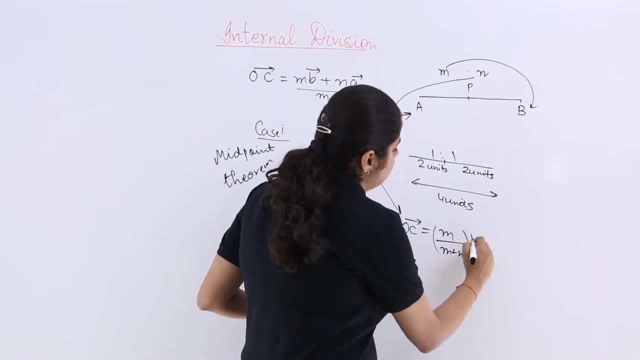 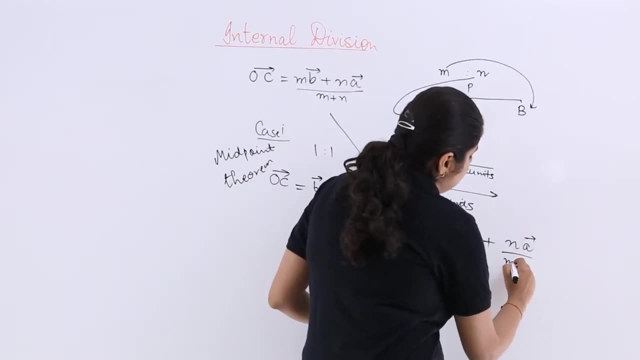 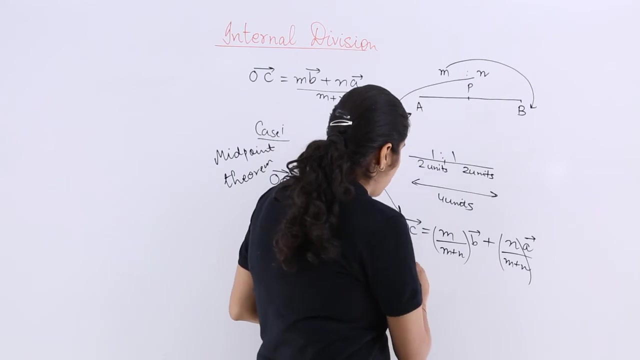 So M upon M plus N multiply by B vector plus NA vector upon N plus N, N multiply by A vector upon M plus N. Now see, this is again very important- OC vector will be what B vector and A vector are separate If I write it as lambda: A vector plus mu A vector.